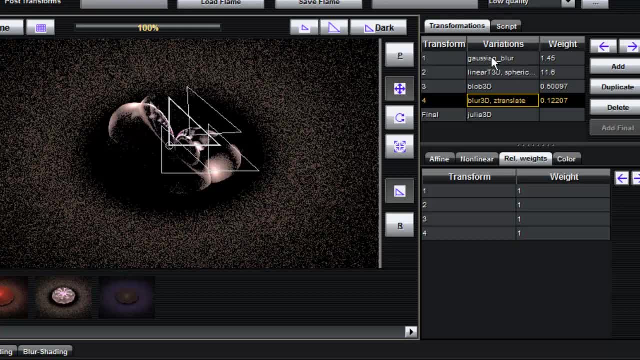 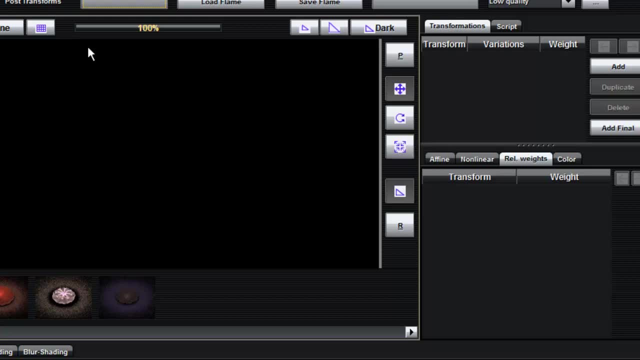 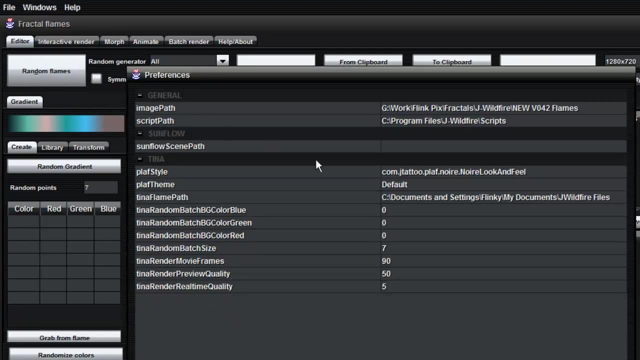 in the early days here and just get you going. So what we're going to do here is we're going to start up and show you a couple of things. First of all, the random flame generation, And one thing that you can do here is, if you go to the preferences, 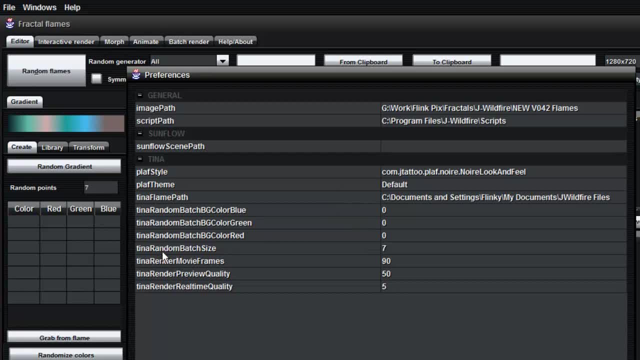 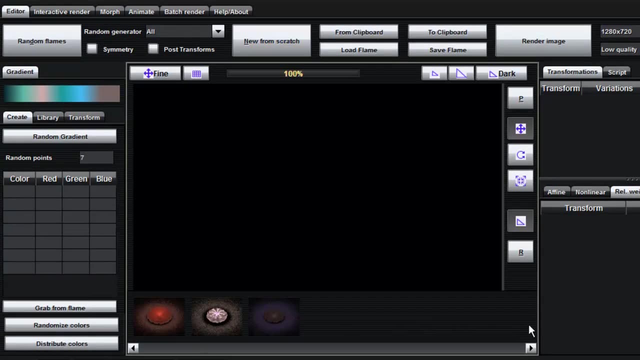 you'll see here that under TINA, random batch size, I've set that to seven. It's standard defaults to 24, which is a lot of randomly generated flames And you're going to be. you know, given the whole rake of them down here, Seven is exactly what fits in my particular viewport, or in my particular. 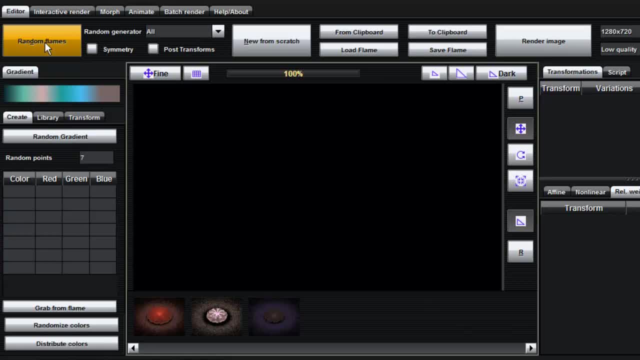 setup down here. So if I want to sort of create a set of random flames, all you have to do is decide which type There's: bubbles, bubbles, three-dimensional ones and experimental 3D gnarles. experimental gnarles, flowers, 3D stunning. 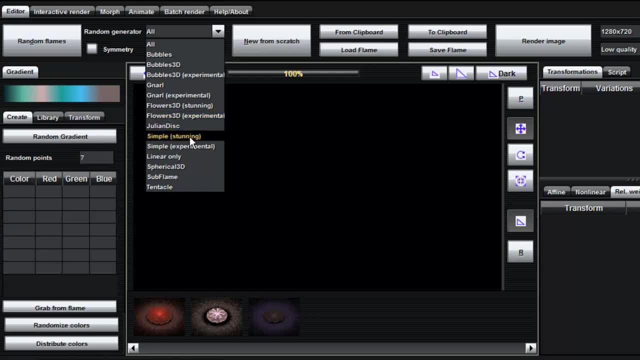 ones: experimental flowers, Julian discs, simple, simple, experimental, linear, only spherical 3D sub flames and tentacles. Now, if you leave it at all, it'll then give you a random collection of all of these. So by clicking random flames you can see here as it's creating these. 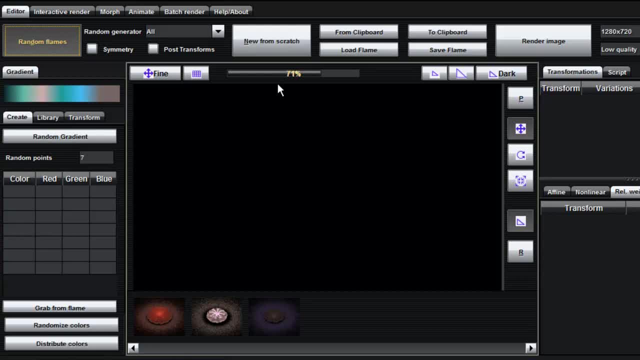 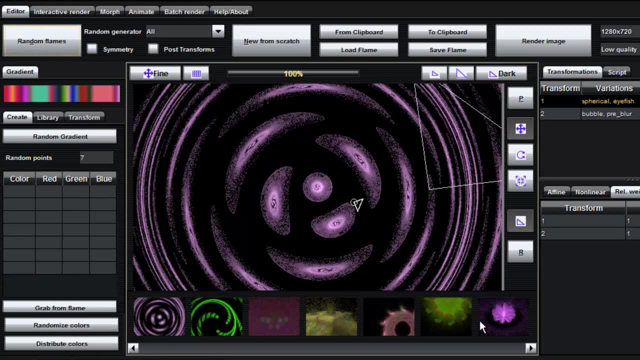 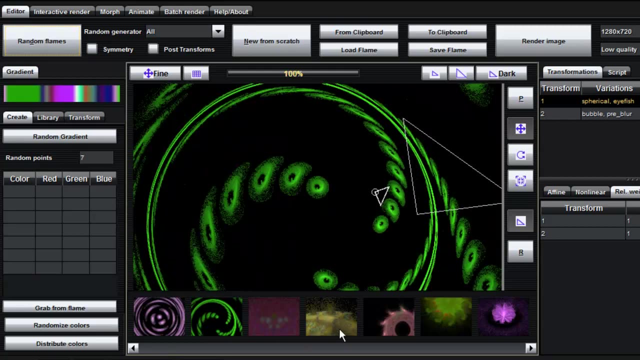 you get a progress indication while they're being produced. And there we have it. I have now seven new randomly generated flames and you can just basically see what they look like. Just double click on each individual one and have a look and see what you like, If there's anything there that you kind of want to see. 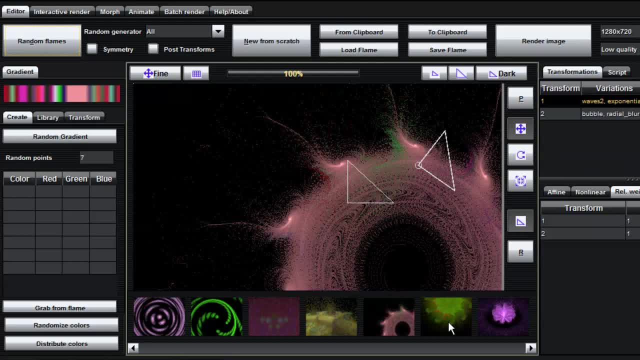 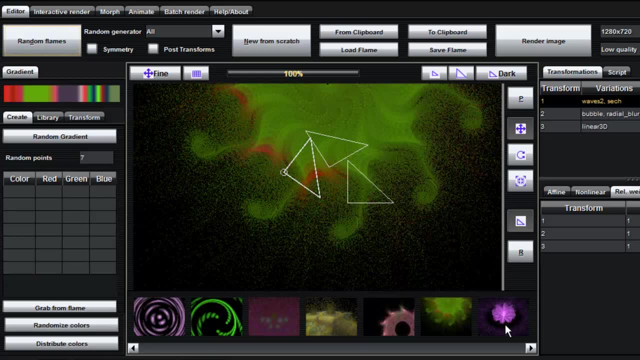 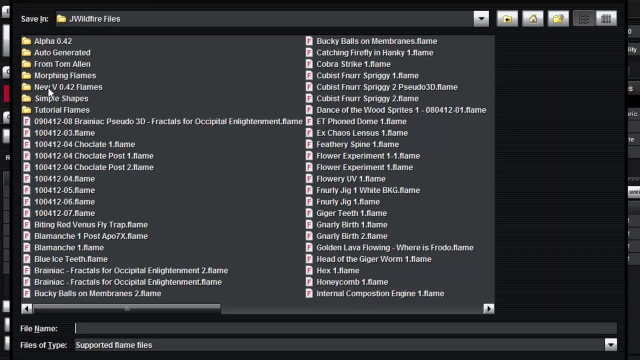 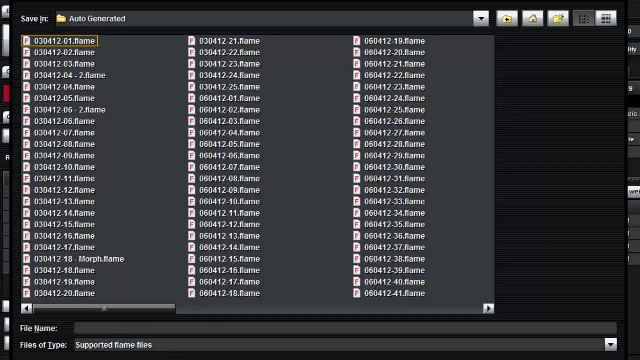 that you want to play with, go for it. And perhaps, before you start messing about too much, you might want to just save the flame, And in my case, what I tend to do when I save flames is I just go in save flame- auto-generated, and I tend to name them according to the date, And today happens to be the 15th. 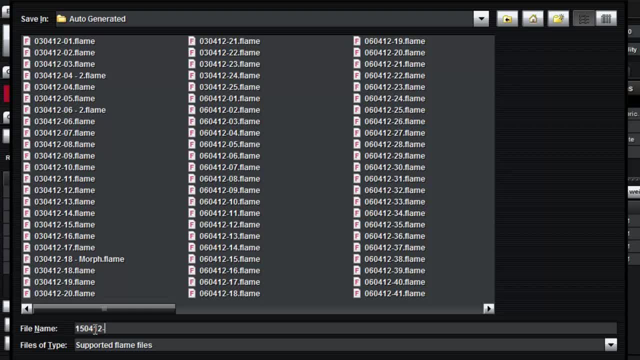 of April 2012.. Put a little hyphen there and start off with 01.. Now, in order to sort of save them quickly, I tend to select that and do control C to save that, so I can remember which number I'm up to. 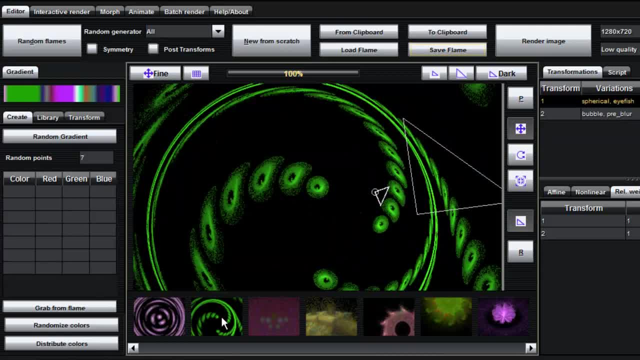 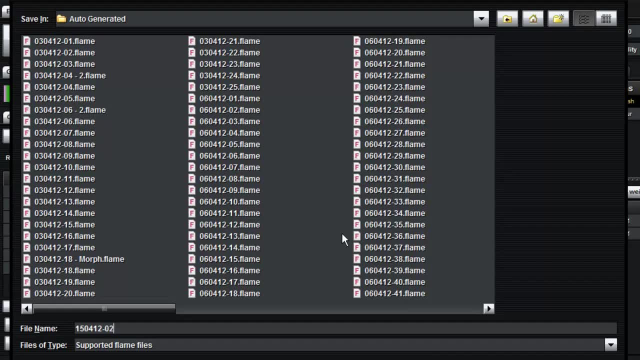 if I'm going to save a lot of them. So I'll just take that one and that one and then I'll put that one in Just control V here, in this case to call that back Shift home control C. so I remember that one. 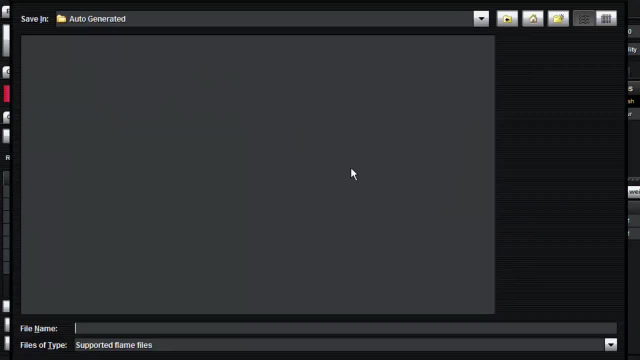 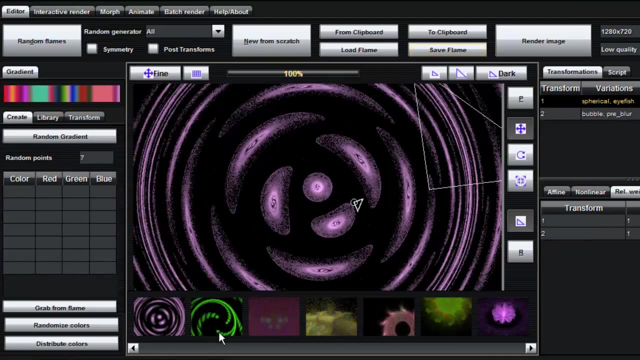 And so on and so forth. so that's just a little quick trick to remember where you are in the numerics You can use copy and paste. Now I've saved three of them. Okay, I'm not happy with most of that. 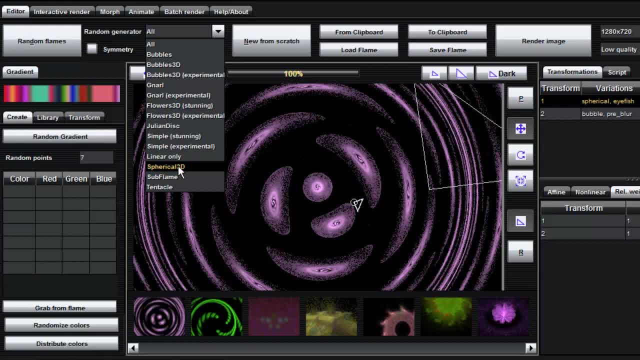 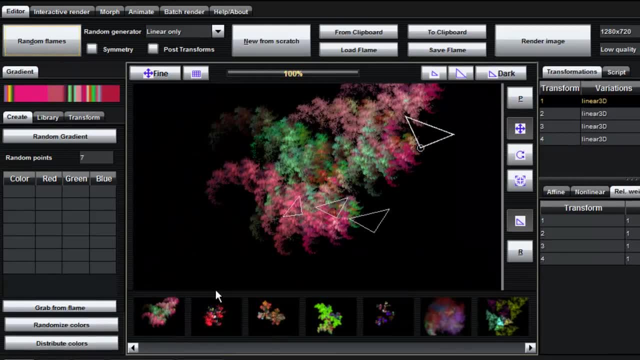 so I'm just going to try a few specific ones like simples or linear only. Click on random flames again and here we have a new batch with linear transforms only, and you can see which ones in fact that's been saved. 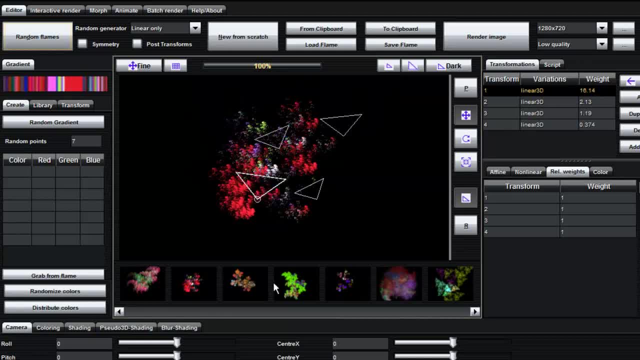 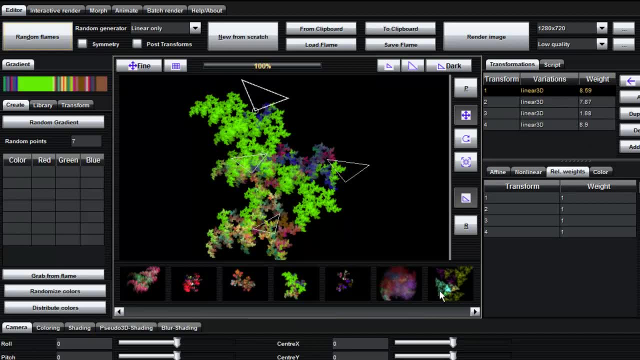 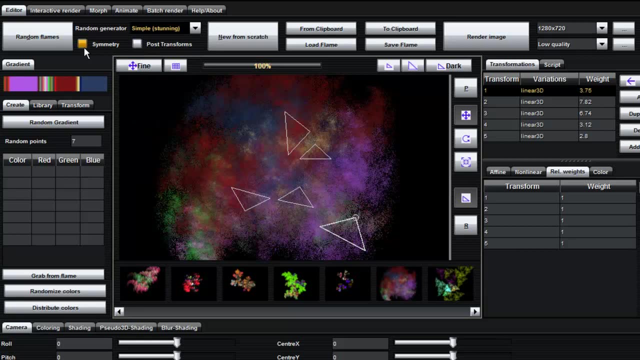 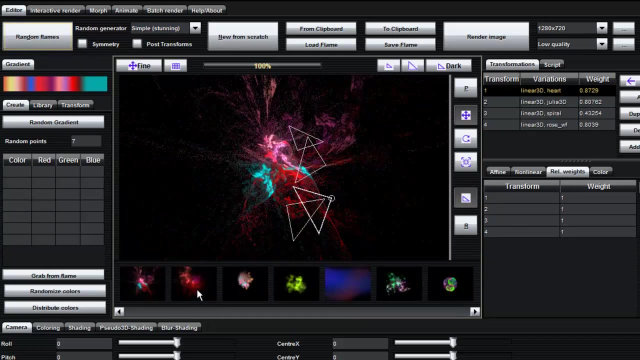 only, and you can see which ones are applied on each days and if you like anything and just save it, the simple ones are quite cool, simple, stunning. you also have two options here- symmetry and post transforms- and we're gonna just do a quick random again here. okay, so this is what we get with, just simple, stunning. 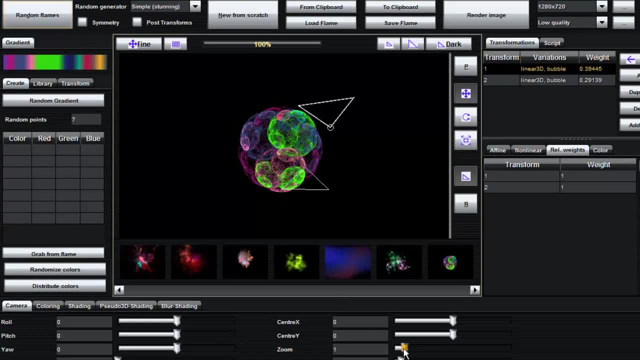 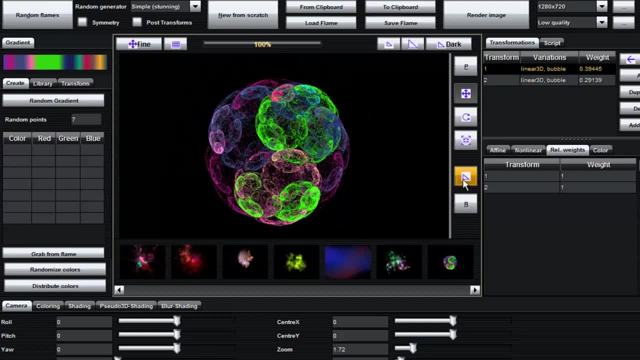 there's an interesting one and before you sort of decide to save them, you might want to zoom in to them a bit. you know, have a look, maybe do a quick without the actual triangles. so I switched off the triangles from you and do a quick render. see what it's like. if I'm happy, I'll save it, if not, I'll go on. 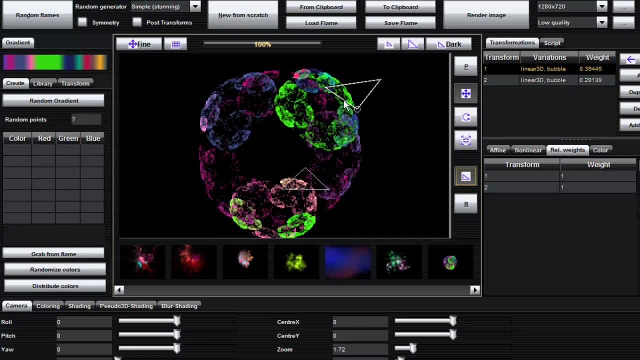 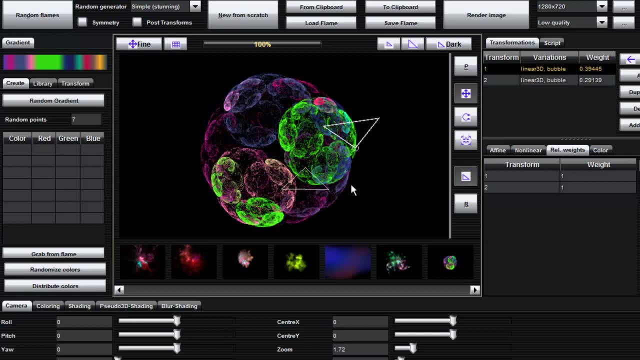 or I might just have a little pool around and play around with these things and, as you can see, it's so easy to just start from something very simple that you got for free start messing about. you can either click on these triangles in here to select them, or you can just go over here to select the individual ones and the 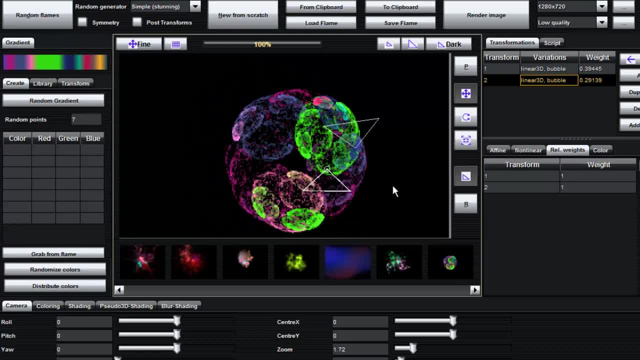 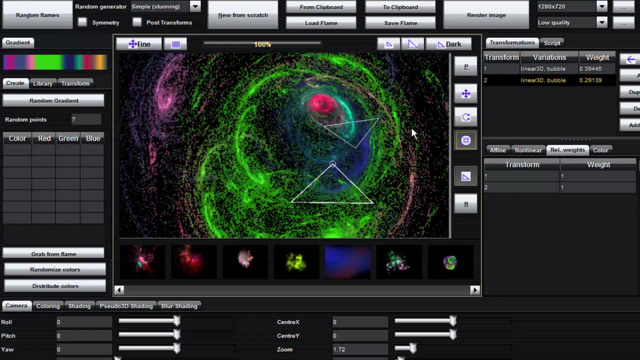 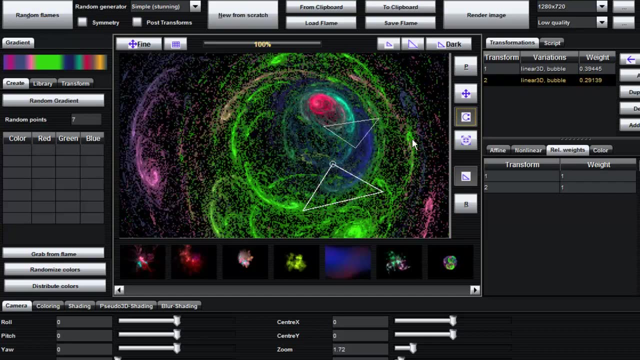 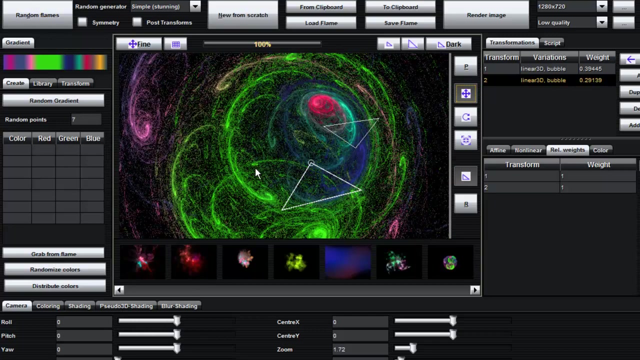 ones that are being pulled, or the transform that you're actually affecting is the one that you have selected up here, and by just kind of scaling, rotating, playing around you very quickly, can create completely different looks of what you were given. so that's a very quick trick. start off with simple, random ones and play around with them and see. 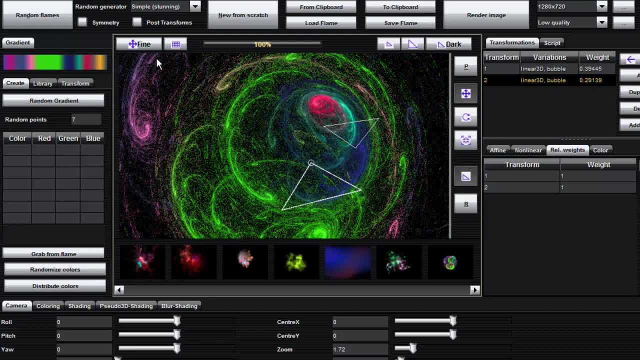 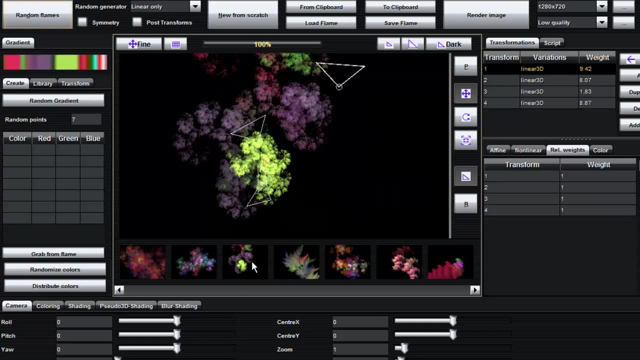 what happens. we'll go into more detail here in a second. now to show you the difference that symmetry does, we start with some linear onlys, do another quick one. you can see that these are fairly random and this is not that much symmetry to it. so if we then just select symmetry and do it again, 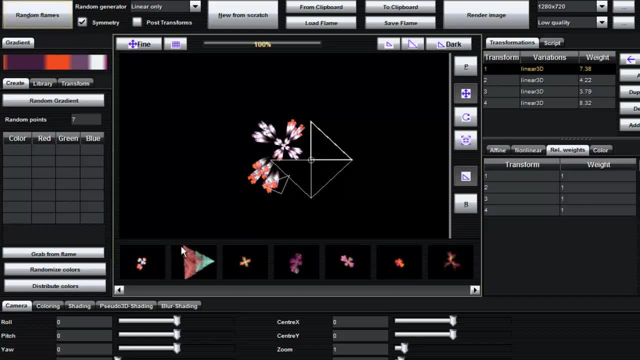 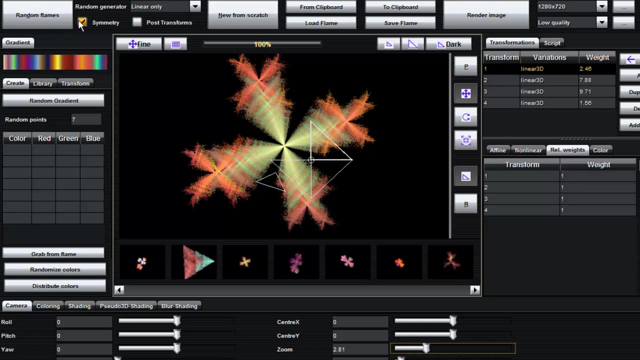 now we look at those random ones, you can see fairly quickly that we have symmetry on the old triangles. here the transforms- this one is quite obvious and, as you can see, you get more symmetrical flames out of those settings. so that's symmetry. and post transforms is when you actually have. 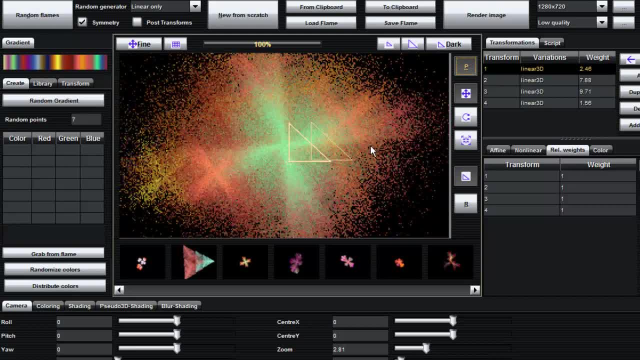 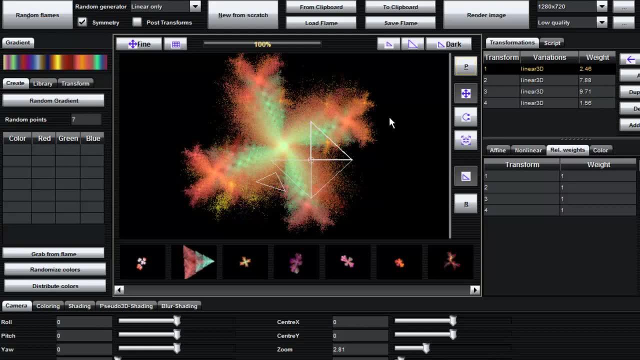 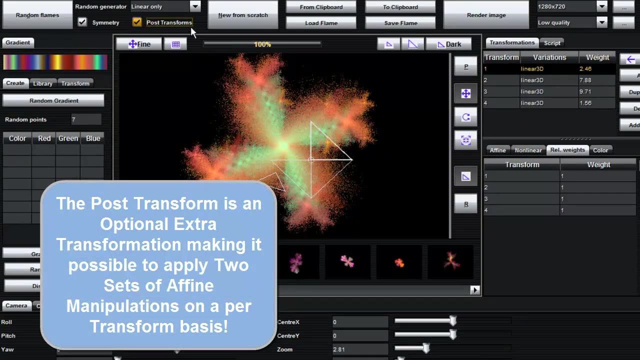 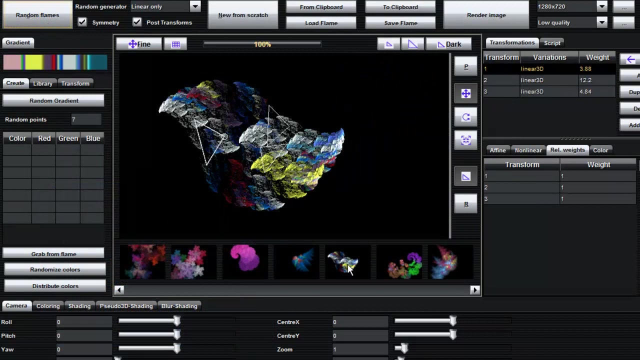 additional transformations applied on a per transform basis now. so there's two parts to any given triangle. there's a post transform and a standard transform. so to just illustrate that, we're going to switch on post transforms and do another random batch and if we look at the post transforms now, you'll see that 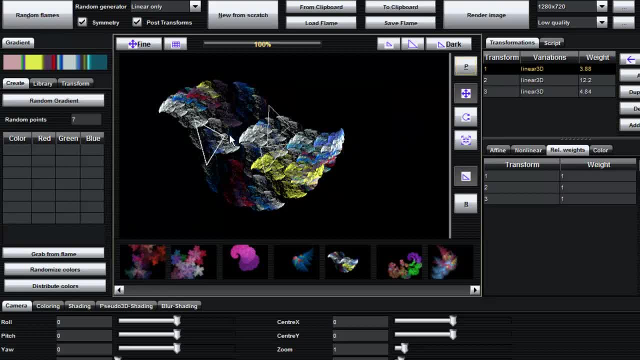 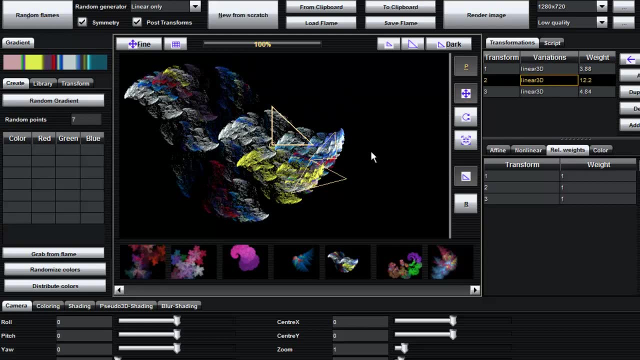 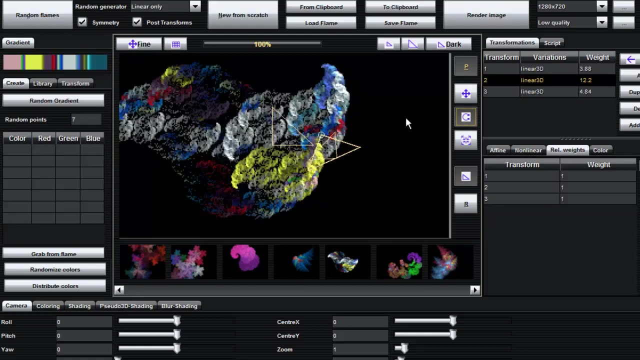 they're in different positions, so they've been shifted from the original transform and that means we get kind of more interesting kind of patterns here. well, not always more interesting, but it's just one additional set of rules and permutations that you can apply to each individual transformation. finally, a 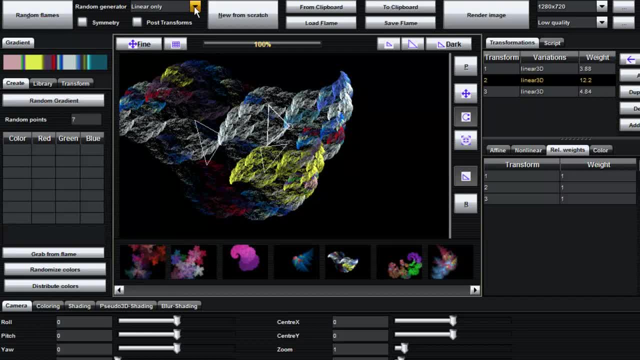 while we're on the random flame generation, and I'm just going to show you an interesting one here: sub flames. now, this is something that we'll go into in a more advanced tutorial in the near future, but sub flames is one very clever trick that JJ wildfire has up its sleeve where you can attach and actual flames.